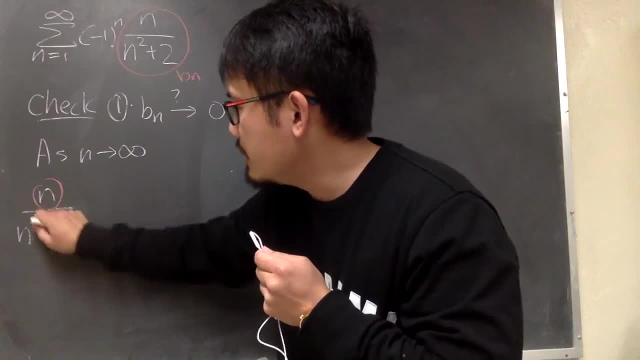 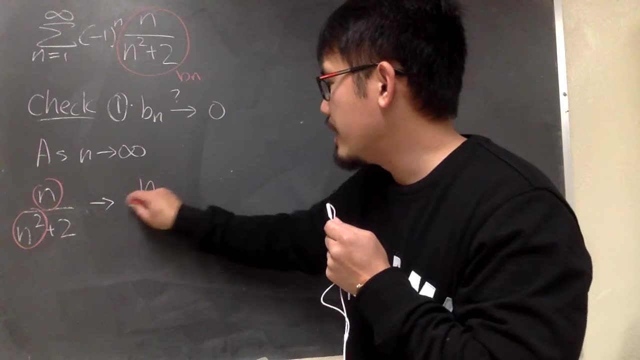 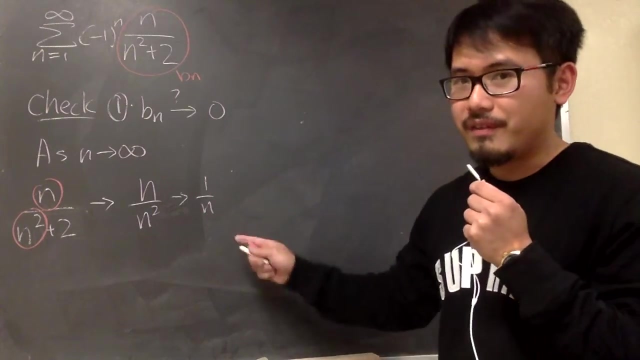 And as n goes to infinity, we know we can just care about this over that. So this is approaching to. so let me draw an arrow. This is approaching to n over n squared, which is approaching to 1 over n, And as n goes to infinity, this is 1 over infinity. 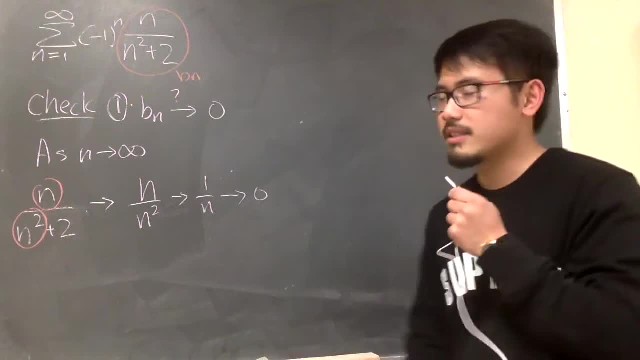 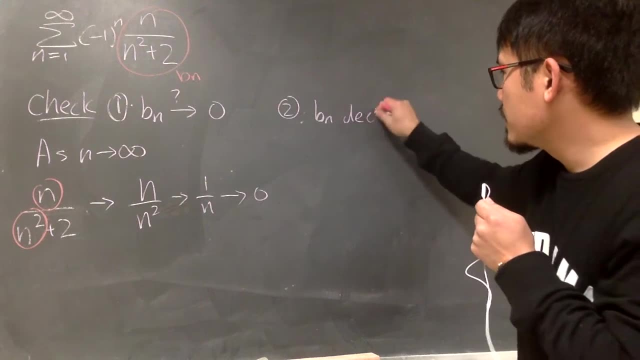 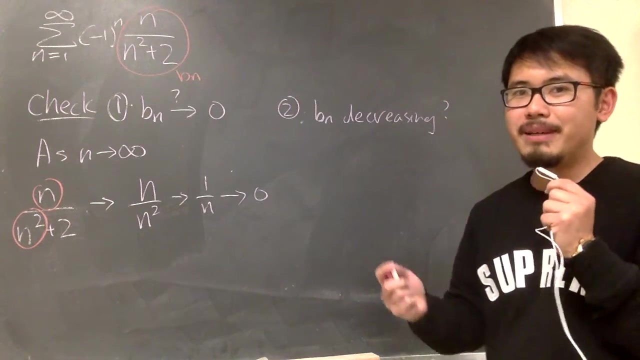 Which is 0.. So, first thing, checks Now. secondly, I want to know if bn is decreasing or not. And now this is the slightly harder part. It depends on your instructor. For my class I will let you guys do this. 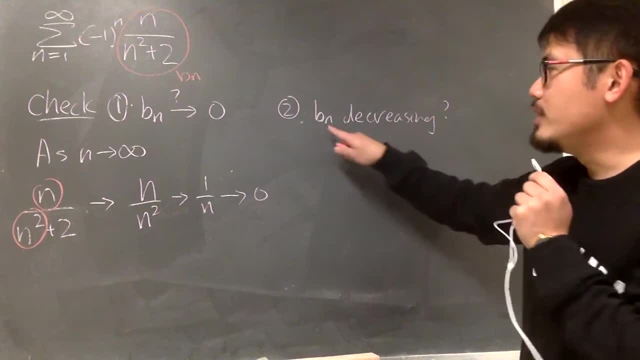 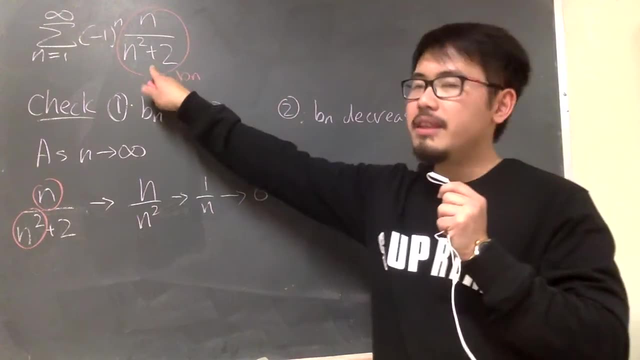 It's okay. All we need is we need to show bn is a decreasing sequence after some n And value. What you can do is look at this and then graph it. Graph the function x over x squared plus 2.. 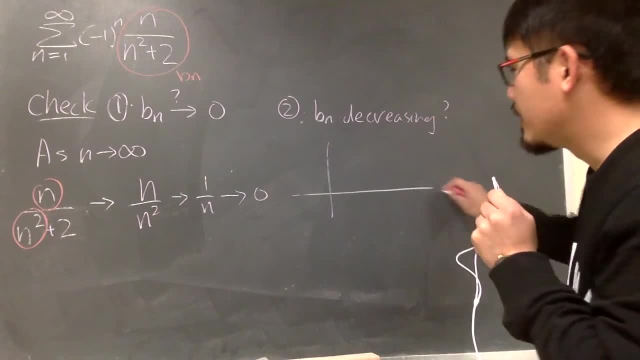 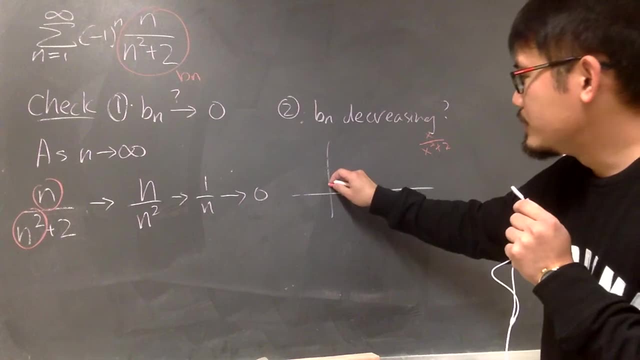 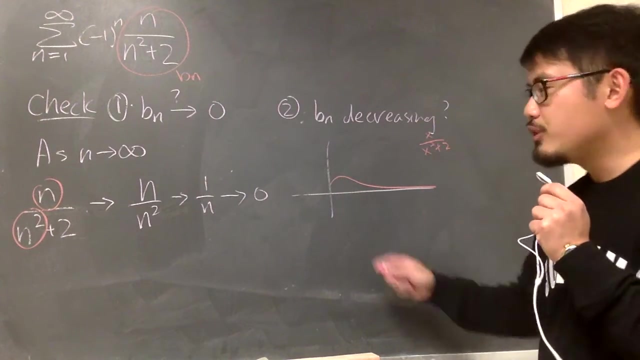 Let me show you the graph. If you want to graph x over x squared plus 2, you are going to end up with something like this: Okay, It is decreasing. And you may be wondering what's this point? the maximum point. 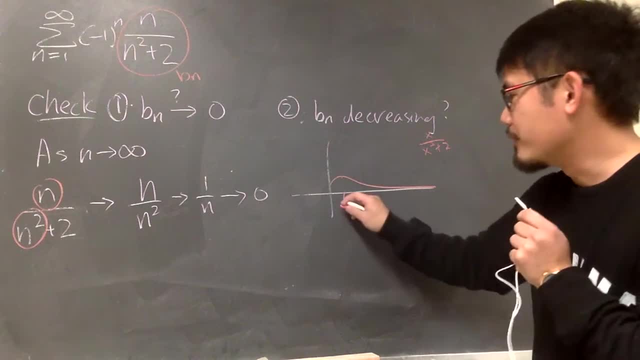 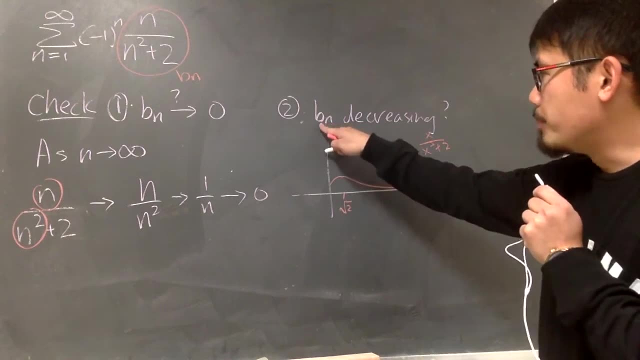 Well, it happens at. x is equal to square root of 2.. Okay, But then all it matters is that you see. the connection of bn and this function is that bn is just the values of this function and the whole numbers. 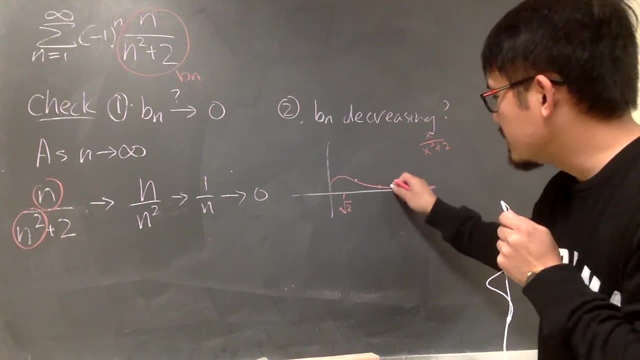 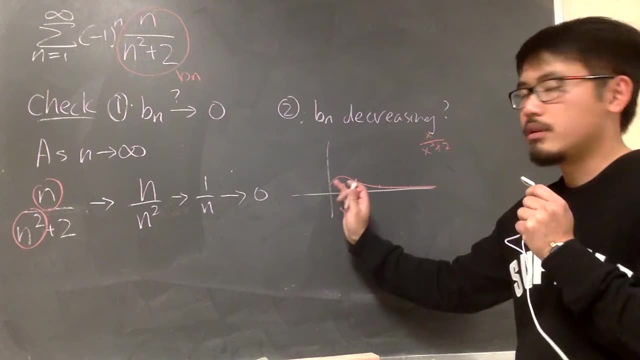 So bn? you are going to just get a bunch of dots on this graph, That's all. bn is decreasing because this function is also decreasing after you have the x value squared of 2.. Psh: Decreasing, Decreasing. 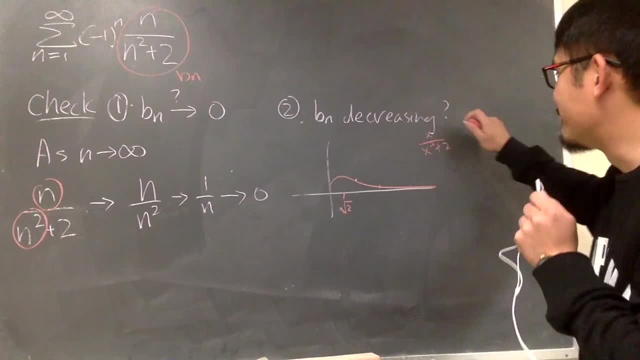 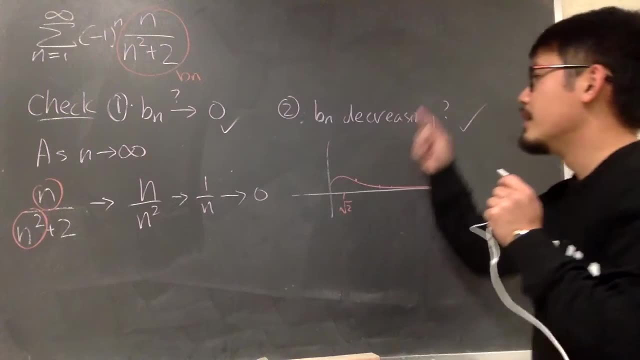 As long as you show me the graph, you are okay. So this part checks. Earlier part checks Two things: bn approaches 0.. And then the second thing is bn decreasing. These are the two things And we just did. 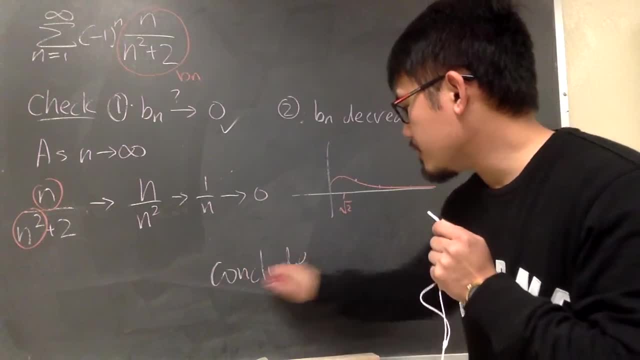 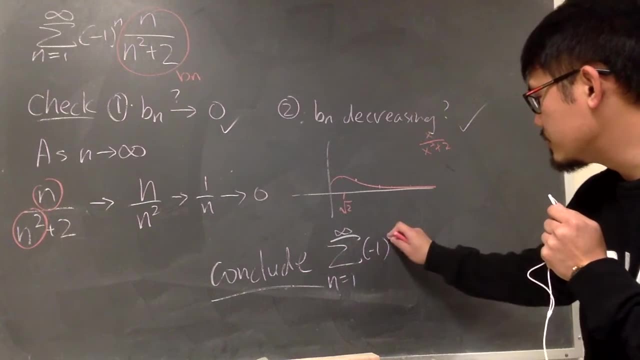 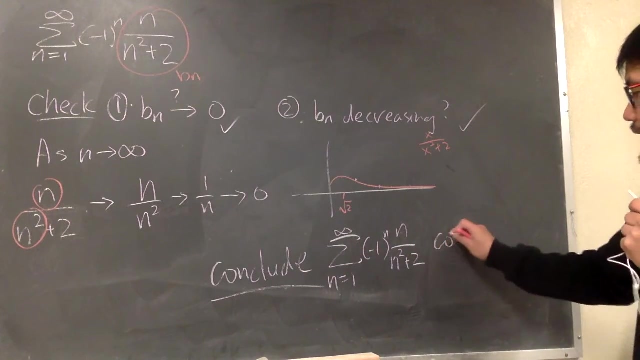 So we can say that Now we conclude The original series sigma as n goes from 1 to infinity negative 1 times- oops, negative 1, to the nth power times, n over n squared plus 2.. This right here it converges by alternating series. test AST: That is it.